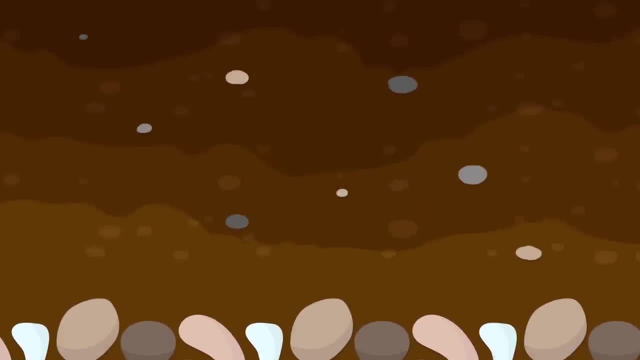 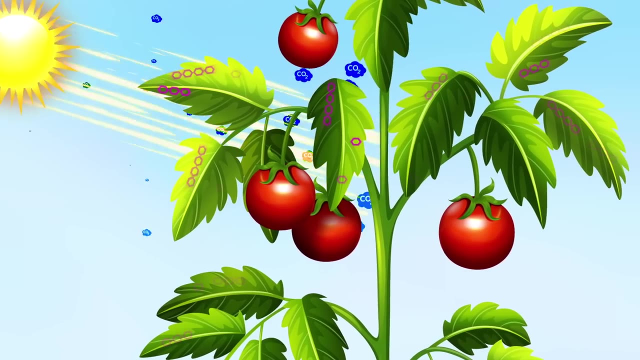 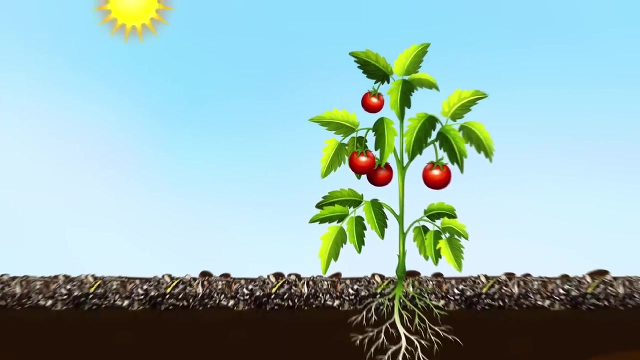 How does nutrient cycling work? During photosynthesis, plants combine carbon dioxide from the atmosphere and sunlight to produce simple sugars and carbohydrates. But, just like humans, plants can't live on sugars and carbs alone. Fortunately for plants, there's a rich source of nutrients right under their feet: in the soil, parent material and in organic matter. 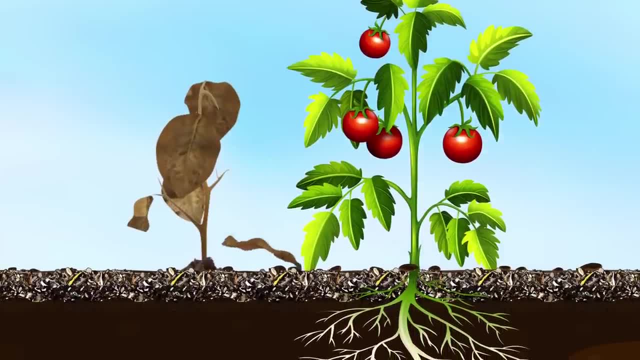 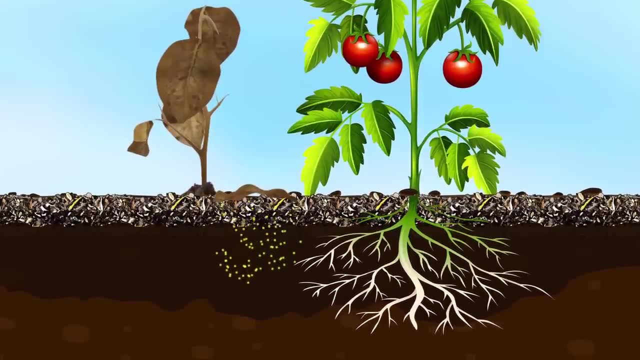 When dead plant material or organic matter falls to the surface of the soil, it's gradually decomposed by microorganisms. Nutrients are then released into the soil in plant-available form. The next generation of plants then absorbs these nutrients, and so nutrient cycling begins again. We humans remove nutrients from this cycle when we take. 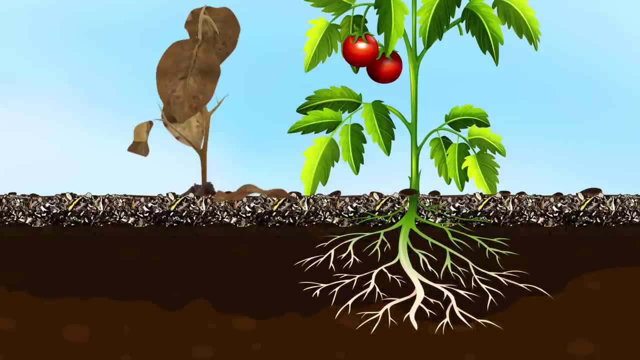 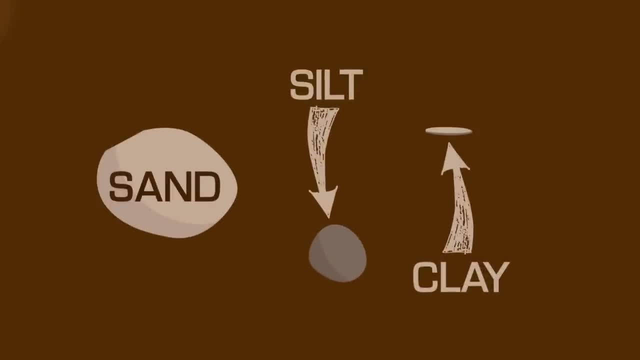 food from our fields, But these are easily replenished when microorganisms harvest nutrients from the parent material: the rocks and pebbles and the much smaller particles such as sand, silts and clays. At the molecular level, the parent material comprises. 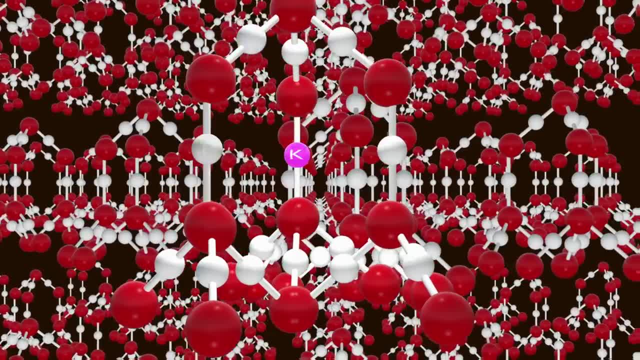 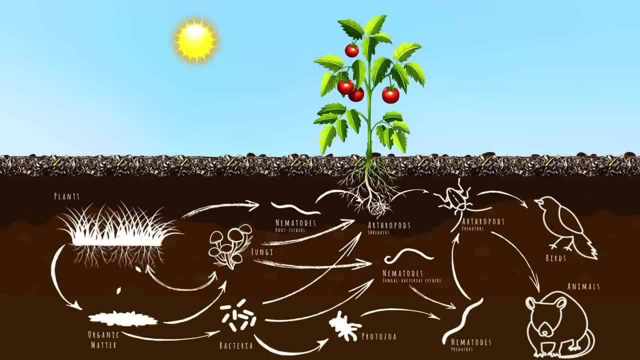 large lattice structures which hold nitrogen, phosphorus, potassium, boron, calcium, iron and all the other nutrients that a plant needs. With a balanced soil food web in place, plants can control the nutrient cycling that's happening in the root zone. 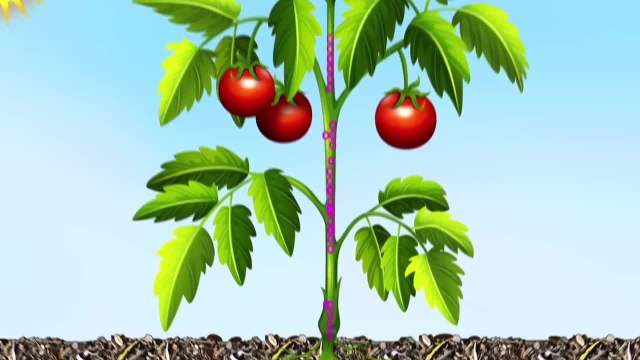 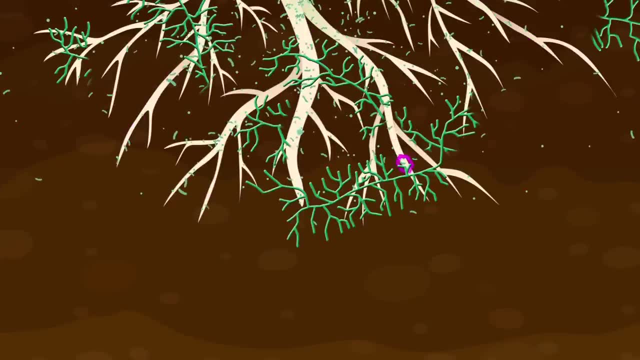 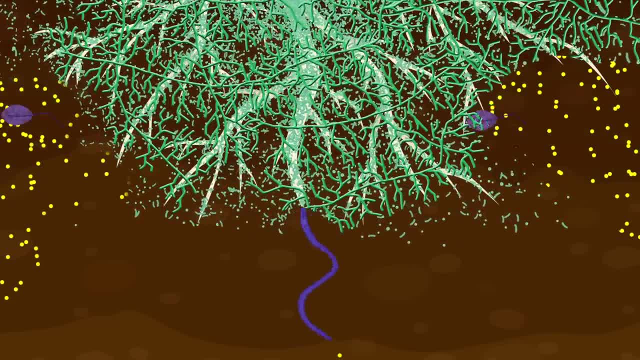 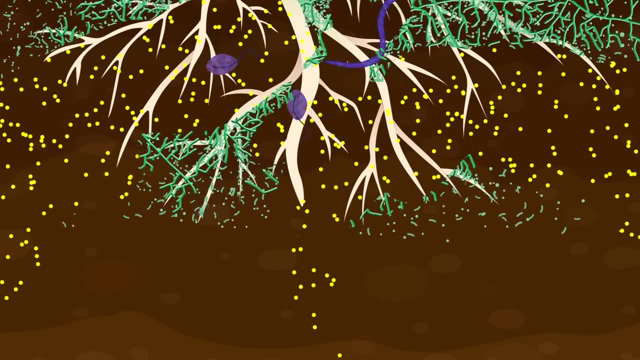 can't live on the soil. So they can't live on the soil. So they can't live on the soil, So they bodies. predatory microorganisms are attracted and they begin consuming the bacteria and fungi. the wastes left behind by these predators contains an abundance of nutrients in plant available form. 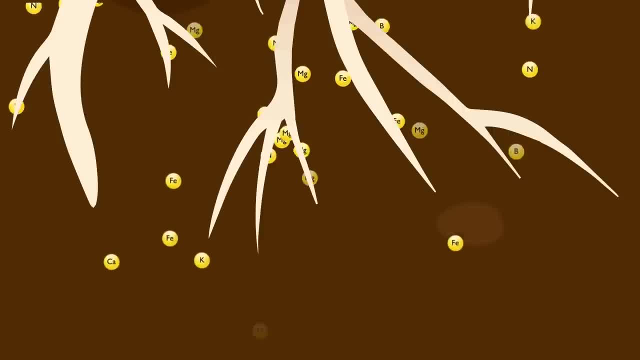 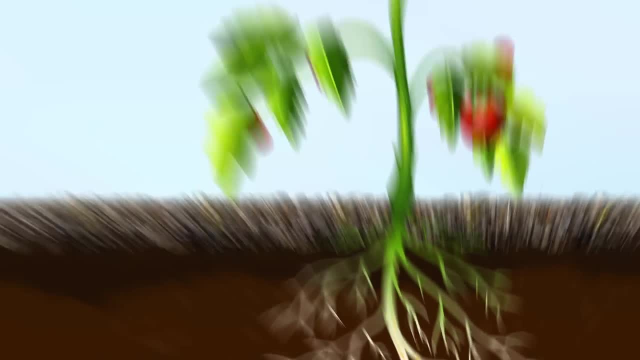 these are easily absorbed into the plant roots, so the plant gets a good return on its investment, exchanging sugars and carbs in return for all the other nutrients it requires. this results in well nourished, resilient plants and in nutrient-dense food for us humans with a balanced soil food web.